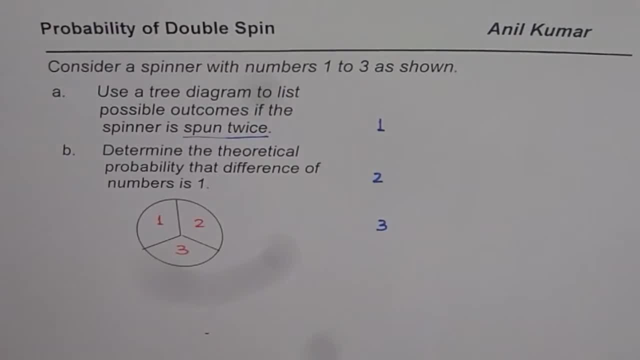 right Now you are spinning it twice, so second time again you could get one, two or three. So in that case, if I have to show it on a tree diagram, how do I show it? So this is the first spin, right? 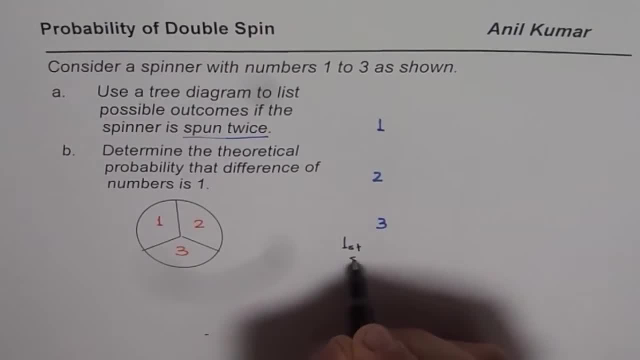 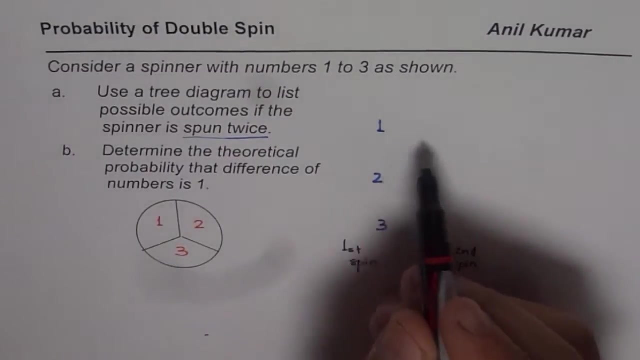 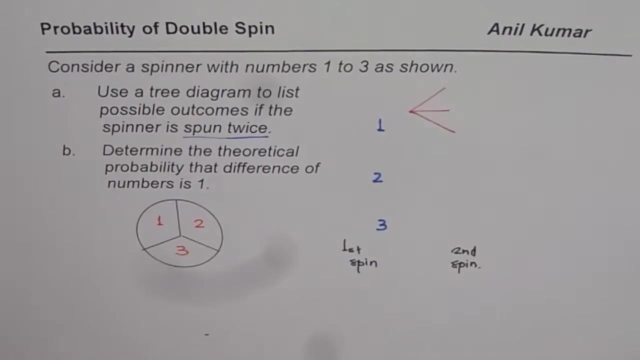 So this is my first spin. Now second spin: what are the chances? Now, let us say, in the first spin we have got one. then in the second spin we could get either one, or we could get two, or we could get three. you get the idea right. 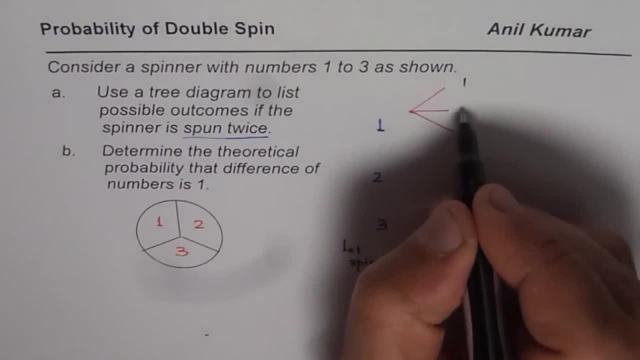 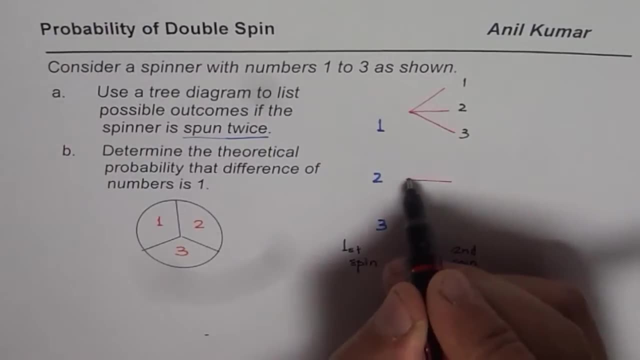 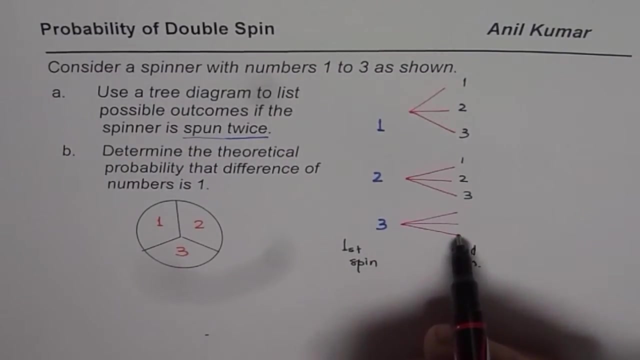 So we could get one, two or three. Similarly, if we would have got two in the first spin, Then also we have the possibility of getting one, two or three right, So we could get one, two or three. For the second spin, again we have three outcomes: one, two or three. do you see that? one, two, 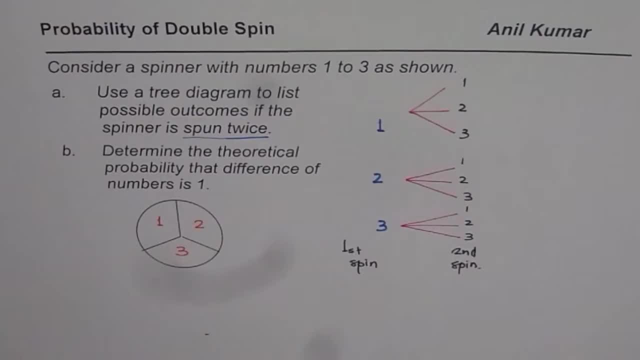 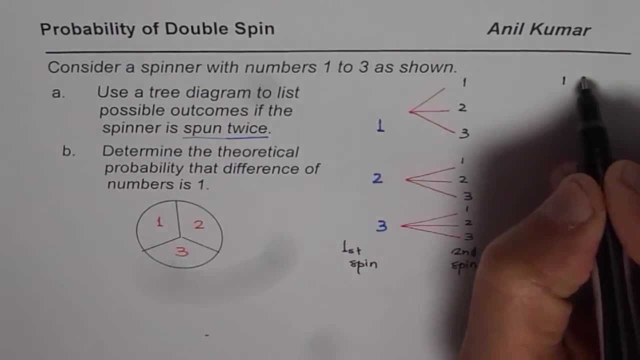 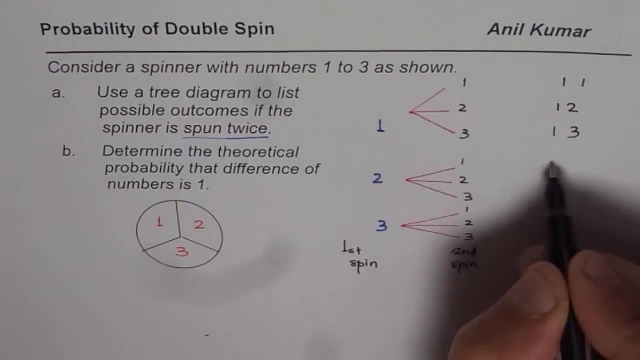 or three. Now, combining these outcomes from the two spins, outcomes could be one one. let me write here: one, one right. One one right Or one two, one two or one three or two. one, two, two, three or three, one three. 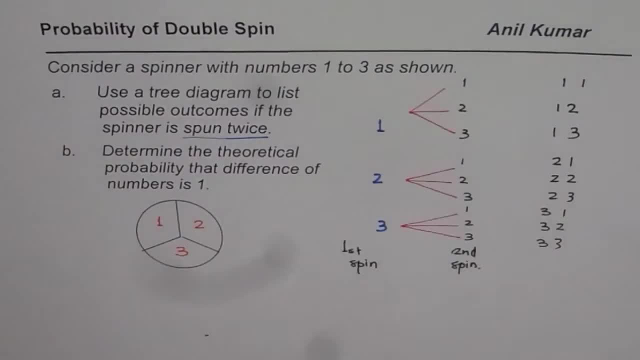 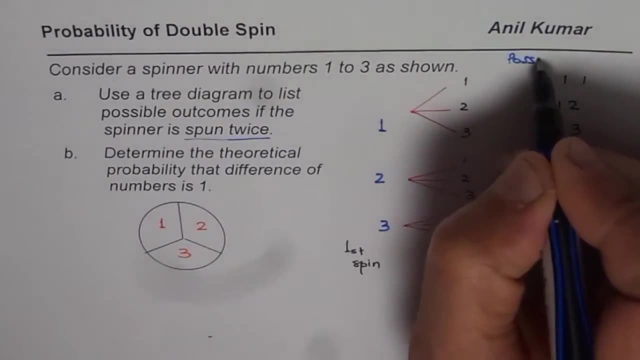 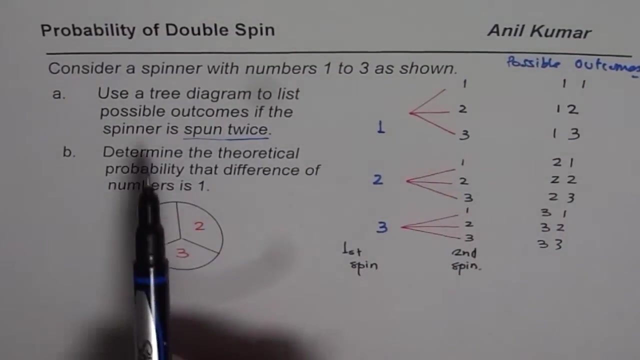 two or three, three. So the tree diagram shows all possible outcomes, right? So these are possible outcomes. So we have done part A, which is use a tree diagram to list possible outcomes. if the spinner has spun twice, Can you tell me how many possible outcomes are there? 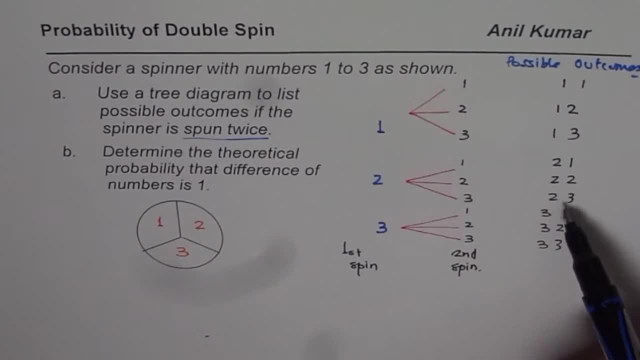 Three times three: nine: one, two, three, four, five, six, seven, eight, nine. So we have nine possible outcomes, right, Nine possible outcomes. Now let's look into the second part of the question. It says: determine the theoretical probability. that difference of number is one. 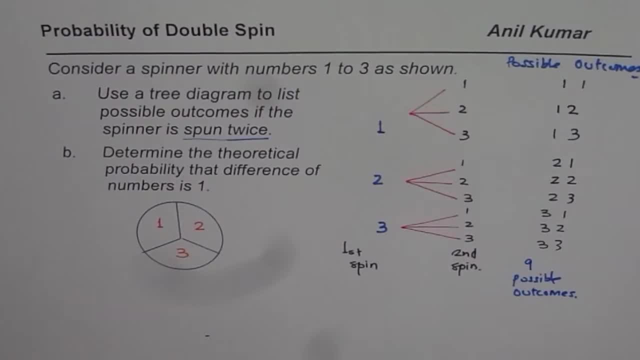 In the two spins we are looking for numbers with difference one. Now there are nine possible outcomes. If I find difference between one and one, it is going to be zero Between two and one. this difference is. let me write difference here. 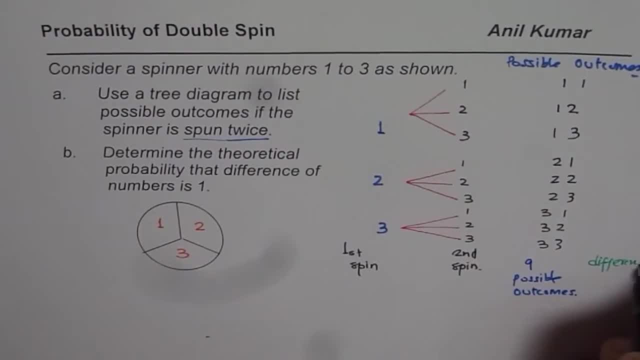 Now let me write difference. Difference here is zero, here it is one, here in this case it is two. Difference here is one. difference is zero. In this case two and three is also one. We can do three minus two. 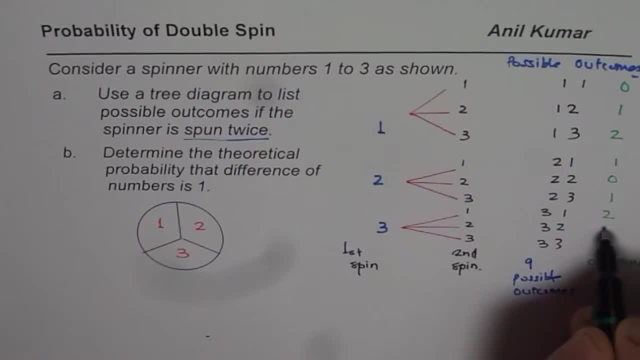 You get the idea right. So three minus one is two, three minus two is one. three minus three is zero. Now in this, how many times do you get difference of one? Let me write it, Highlight those. So four times we get difference of one, correct? 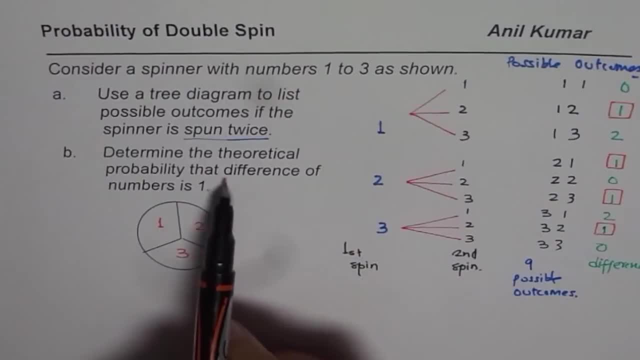 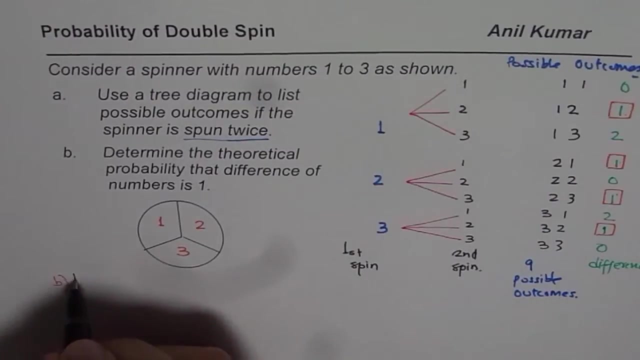 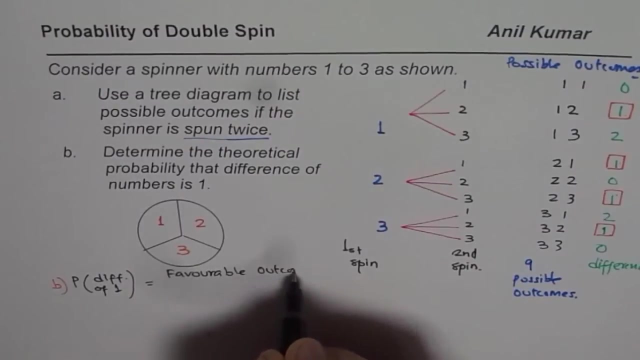 Now the question is: determine the theoretical probability that difference of number is one, So favorable outcomes are one, two, three, four. So for part B our answer will be favorable outcomes, so probability for getting difference of one. So there will be favorable outcomes over total outcomes. 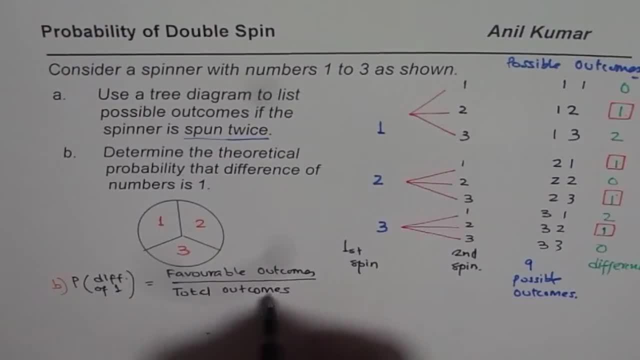 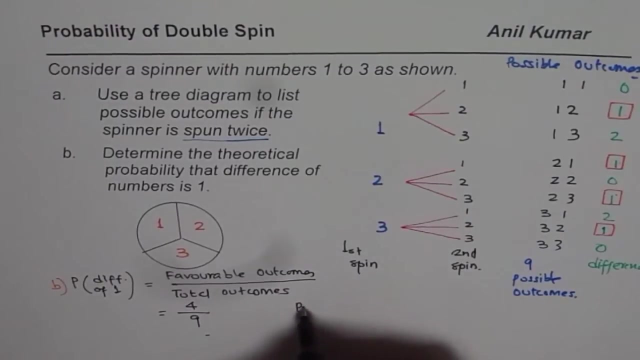 So in our case favorable outcomes are one, two, three, four, So it is four out of total of nine, right? So four out of nine. So that is one way. So that is one way of writing the answer. The other is in percent form, right? 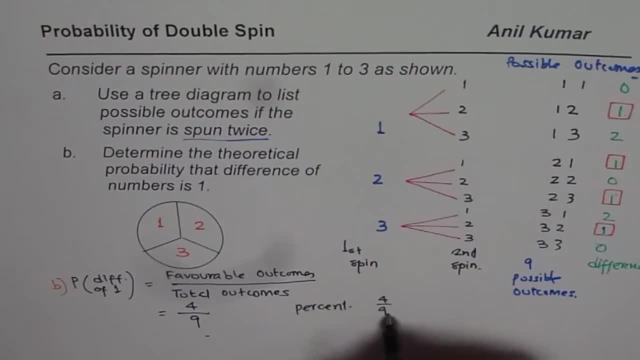 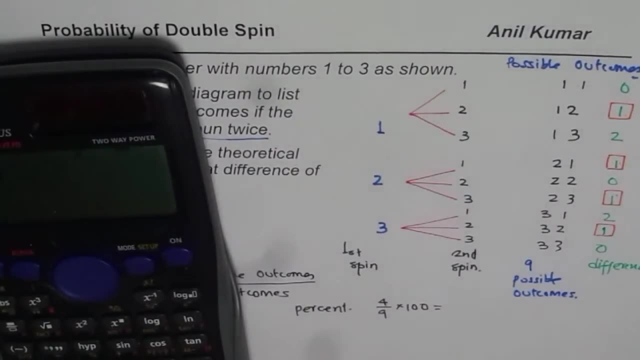 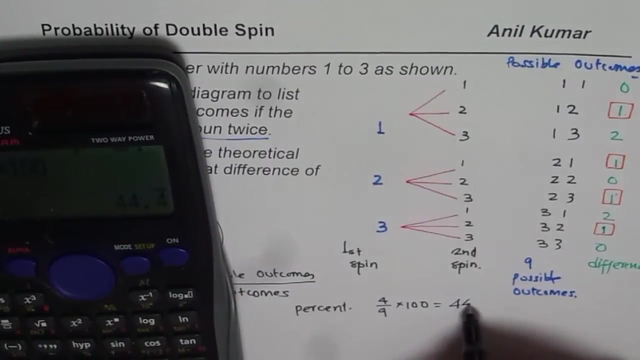 We could also say in percent, that is four over nine times hundred. So let us calculate this also. So we have four divided by nine times hundred, which is 44.4 percent. do you see that? So we could write this answer in percent or in fraction.